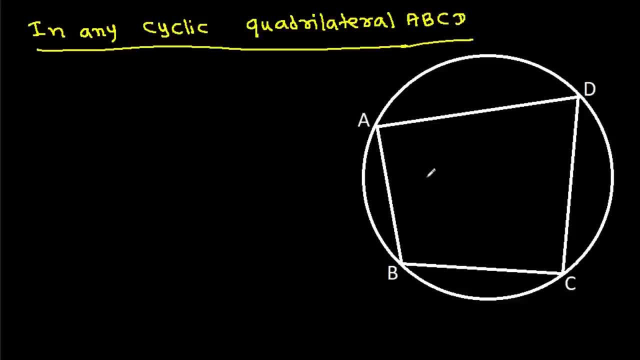 A, B, C, D. if AB is A, BC is B, CD is C and DA is D, Then number 1.. According to Brahmagupta's formula, area of ABCD is A, B, C, D. 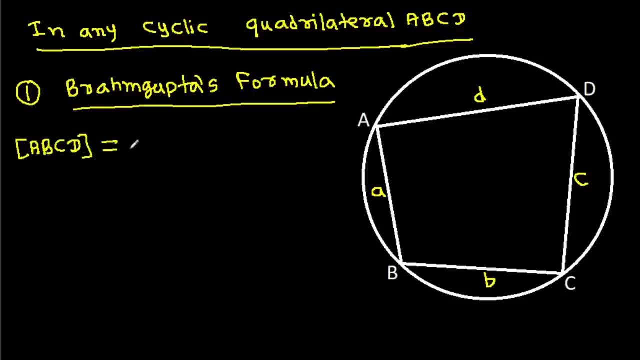 BC is B, CD is C and DA is D. Then number 1.. According to Brahmagupta's formula cd, it is equal to a square root of s minus a, times s minus b, times s minus c, times s minus d, where s it is a plus b plus c plus d by 2.. 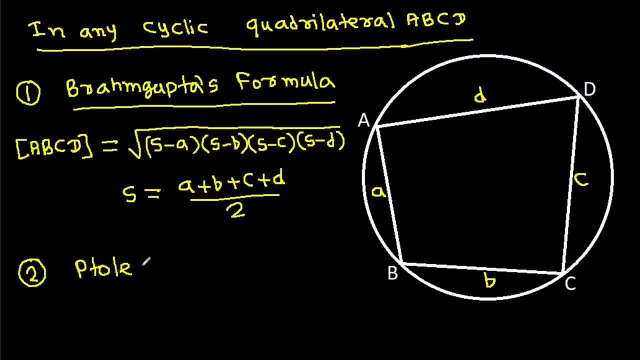 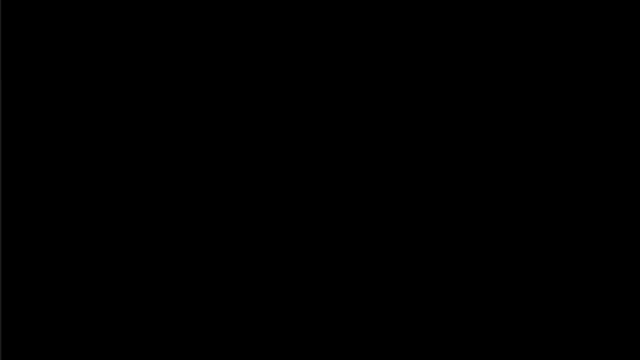 And number 2, Tornomys' theorem. if the diagonal AC is x and bd is y, then according to Tornomys' theorem, xy is y, xy is y, xy is y, it will be equal to AC plus BD. and number 3, in any triangle A B- C, if A- B is A, B, C is B. 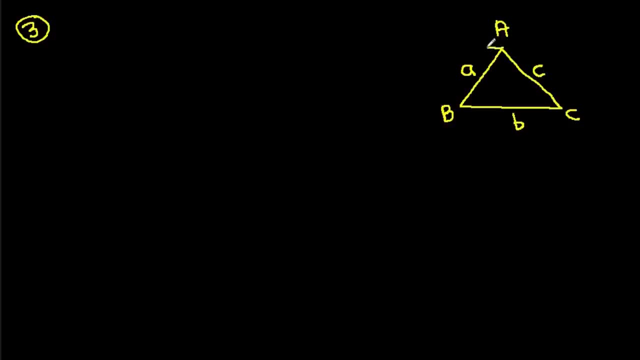 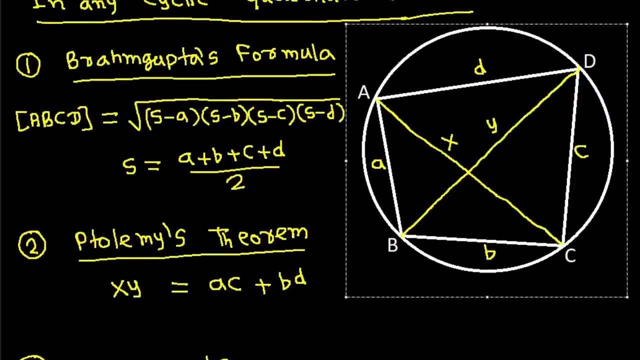 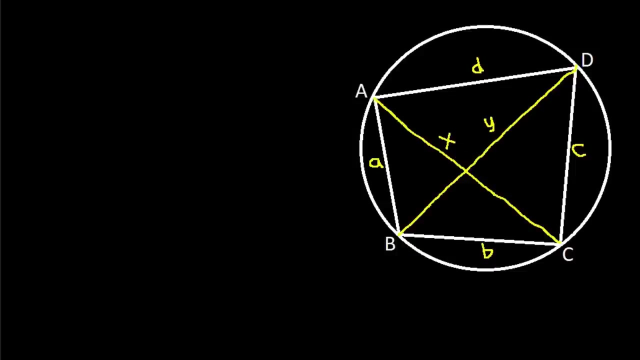 and AC is C, then circum radius R it will be equal to ABC by 4 delta, where R it is circum radius and delta it is area of A, B, C. So here in triangle, A, B, C, A, B is A, B, C is B. and AC is C, then circum radius R, it will be equal to ABC by 4 delta, where R it is circum radius R and AC is C, then circum radius R, it will be equal to ABC by 4 delta, where R it is circum radius R. 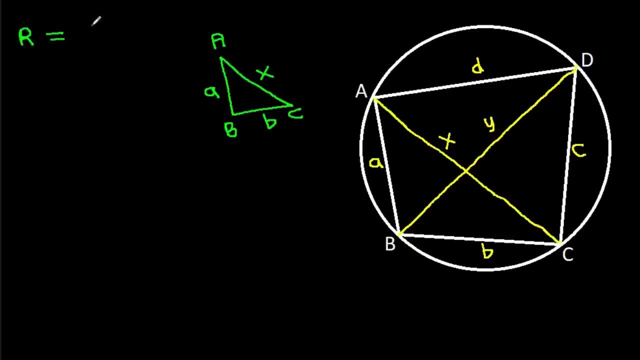 and AC is C, then circum radius R it will be equal to ABC by 4 delta. where R it is circum radius R we have AC is X, AD is D and CD is C. so circum radius it will be equal to CDX by 4 times area of ACD. 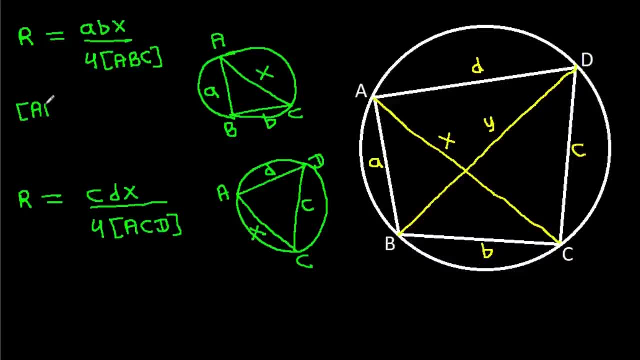 and from here we can get: area of ABC is ABX by 4R and from here area of ACD, it will be CDX by 4R and from here area of ACD, it will be CDX by 4R. 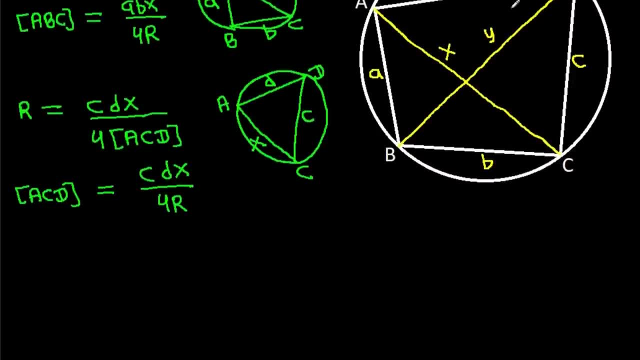 and from here area of ACD, it will be CDX by 4R. and if we add area of ABC and area of ACD and if we add area of ABC and area of ACD, then it will be ABX by 4R plus CDX by 4R. 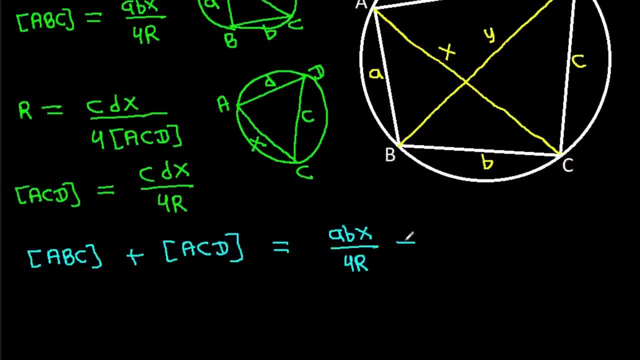 then it will be ABX by 4R plus CDX by 4R plus CDX by 4R. then it will be ABX by 4R plus CDX by 4R, plus CDX by 4R, plus CDX by 4R. 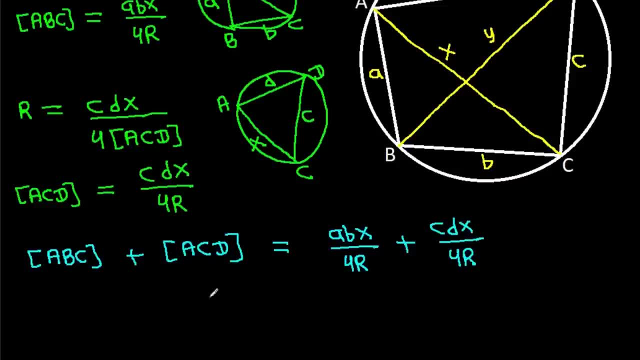 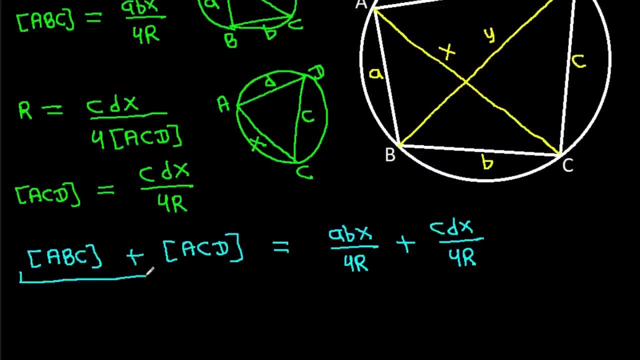 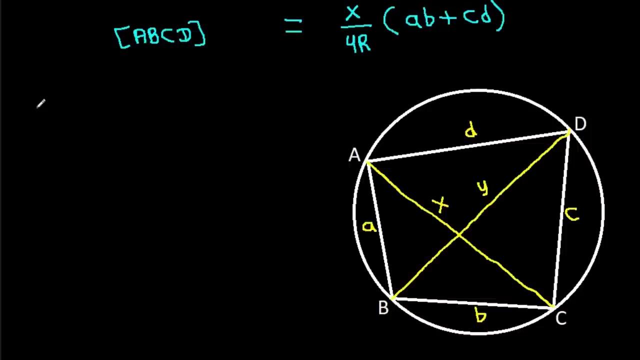 and area of ABC plus area of ACD, it will be area of ABCD. It is equal to. here we can take X by 4R common and it will be AB plus CD. So we get area of ABCD is X by 4R times AB plus CD from diagonal X. 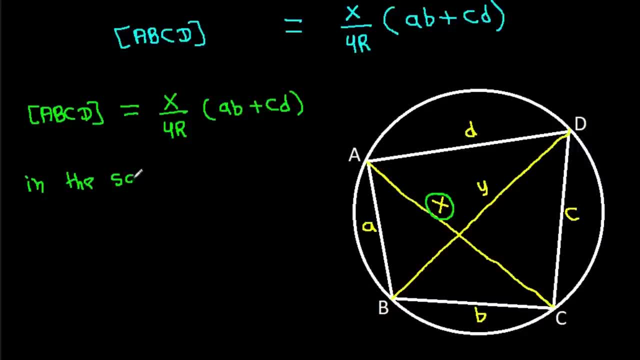 So in the same way, from diagonal X we get area of ABCD is X by 4R times AB plus CD. from diagonal X, Diagonal Y, we can get area of ABCD is equal to Y by 4R times AD plus BC. 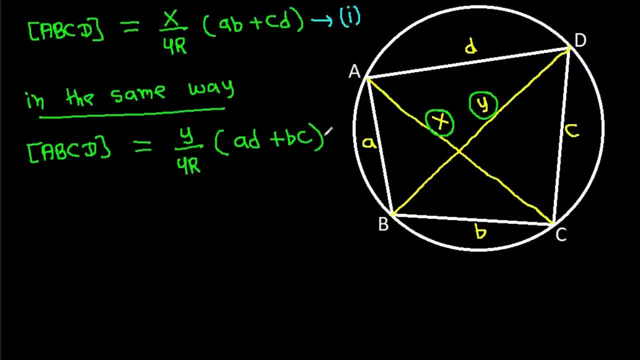 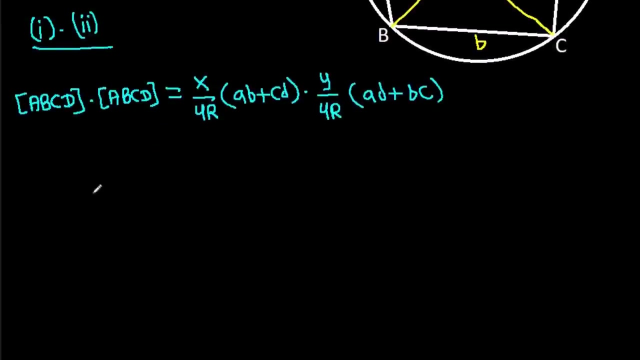 And suppose this is equation 1 and this is equation 2, and if we multiply, and if we multiply equation 1 and equation 2, then area of ABCD times, area of ABCD, it will be equal to X by 4R times AB plus CD times Y by 4R times AD plus BC. 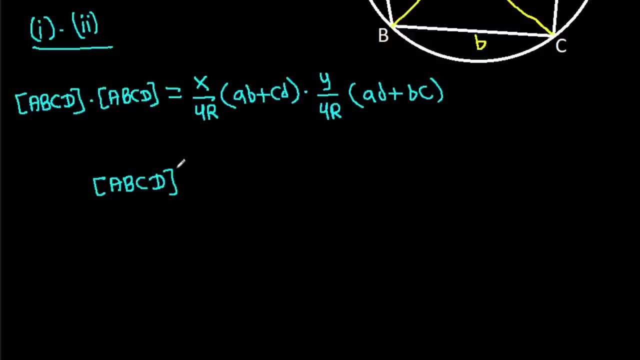 and x dx by 4R times y times AB plus BC. It is area of ABCD square is equal to XY by 16 R square times AB plus CD, times AD plus BC. So R square it will be equal to XY times AB plus CD, times AD plus BC by 16 times area of ABCD square. 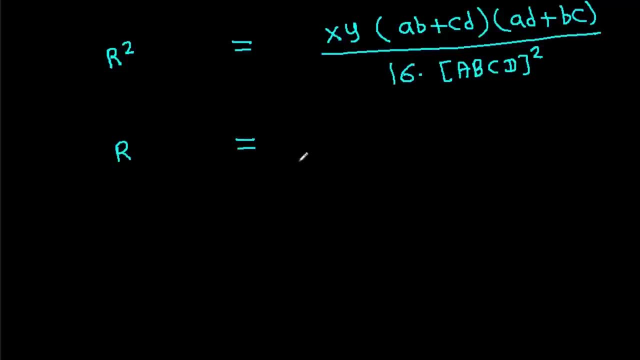 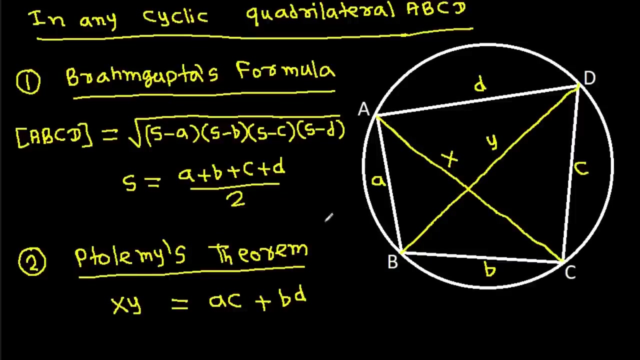 And R, it will be equal to S square root. So R square of XY times AB plus CD, times AD plus BC, by 4 times area of ABCD, And now we have area of ABCD. So R square of XY is S square root of S minus A, times S minus B, times S minus C, times S minus D. 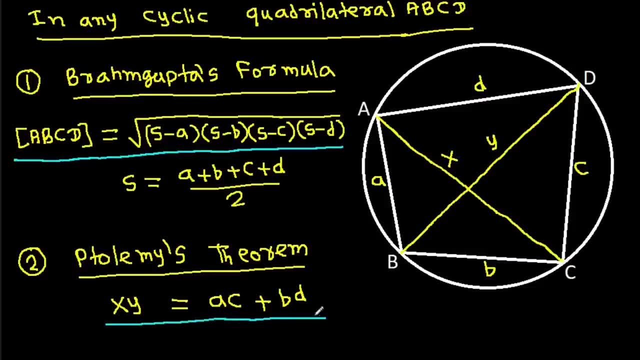 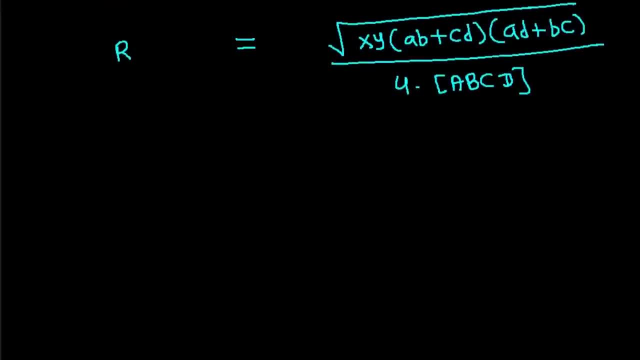 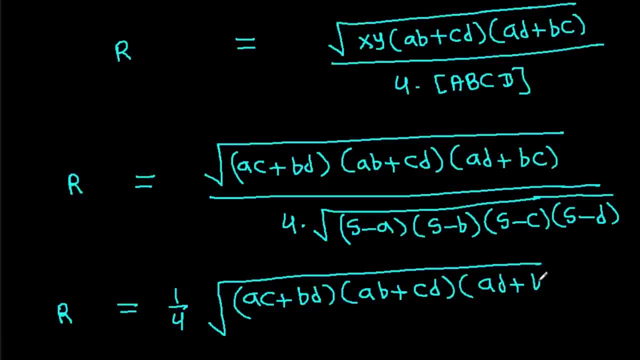 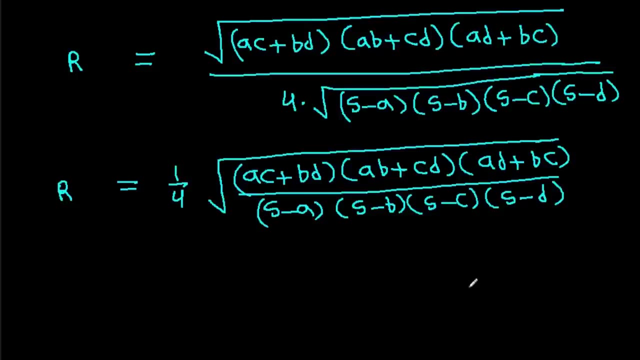 So R square of XY times AB plus CD, times AD plus BC, by 4 times area of ABCD, cd times ad plus bc, by s minus a times s minus b, times s minus c, times s minus d. So r is equal to 1 by 4 times a square root, and this is simply ab, ac, ad and plus cd plus. 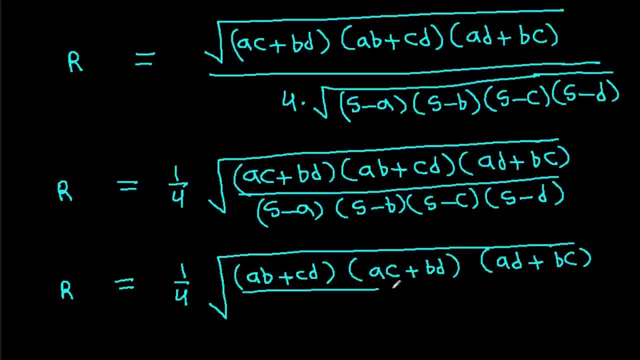 bd plus bc by s minus a times s minus d, So r is equal to 1 by 4 times a square root, and this is simply ab, ac, ad and plus cd by s minus a times s minus b, times s minus c times s minus d. 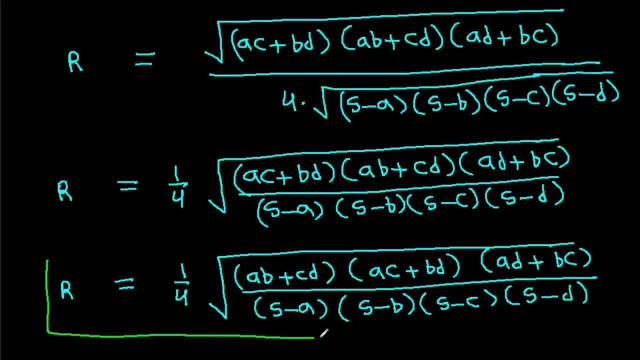 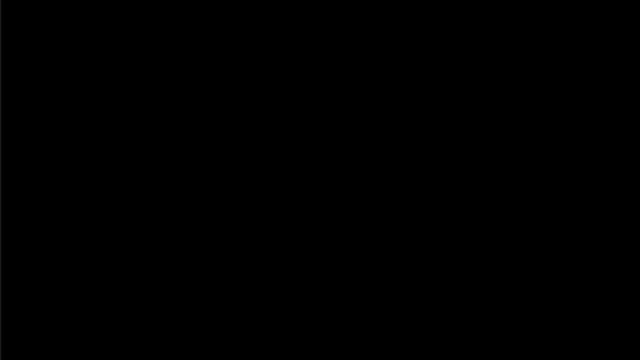 So r is equal to 1 by 4 times a square root and this is simply ab, ac, ad and plus cd, c is 5 and b is 6.. We have: a is 3, b is 4, c is 5 and d is 6.. 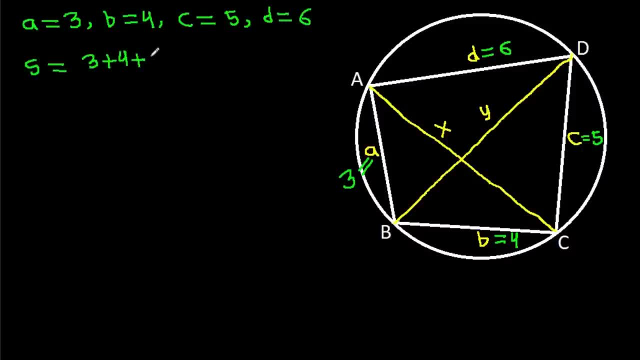 So s it will be equal to 3 plus 4 plus 5 plus 6 by 2, and it is 18 by 2, that will be 9 and r it is equal to 1.. 1 by 4 times s square root of ab plus cd times, ac plus bd times, ad plus bc, by s minus a times. 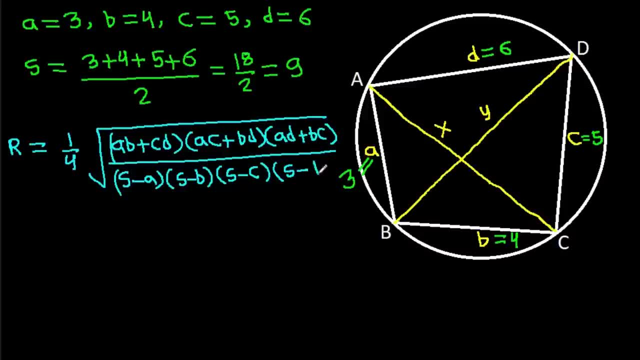 s minus b times s minus c, times s minus d, so r it will be 1 by 4 times s square root, and ab will be 12 plus cd will be 30 times ac will be 15 plus bd will be 24 times cd. 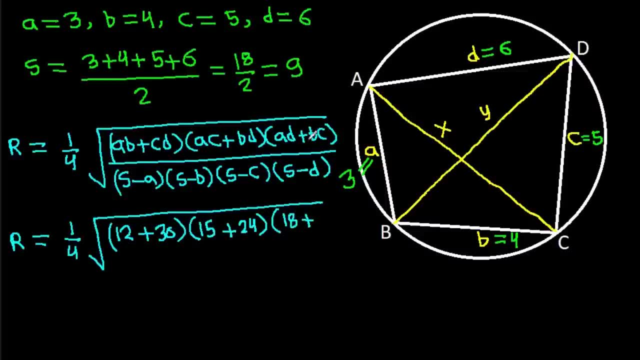 times ad will be 18 plus bc will be 20 by s minus a will be 6 times s. minus b will be 5 times s minus c will be 4 times s minus d will be 3, so r it is equal to 1 by 4 times. 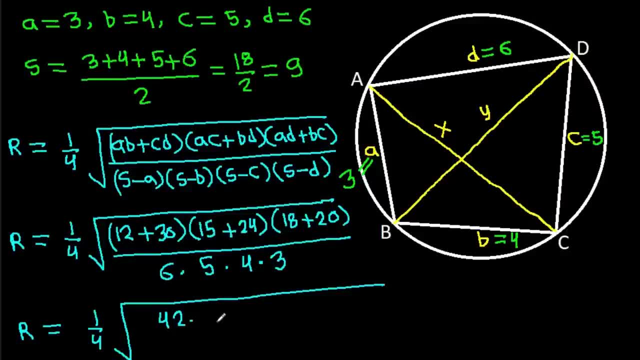 s minus a times s minus r is equal to 30 times 29. pi by 10 s minus 5 is equal to 30 times out is equal to 45 times 16bear aş BERRAT, lemme repeat whether you are reading this as 19, the answer loosen. so 3 divided by 2, that is your stress. 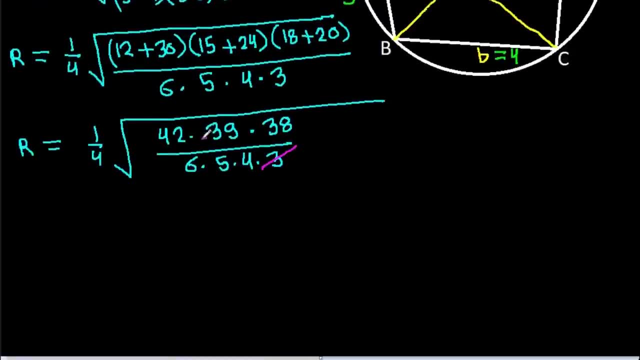 stress values, just like that, for all these different signatures of the index. your where there is going to be Home. 4 multiple升 from the sign of the 4th hand comes from the 3rd by 6 times 4, the next cd times s minus b. 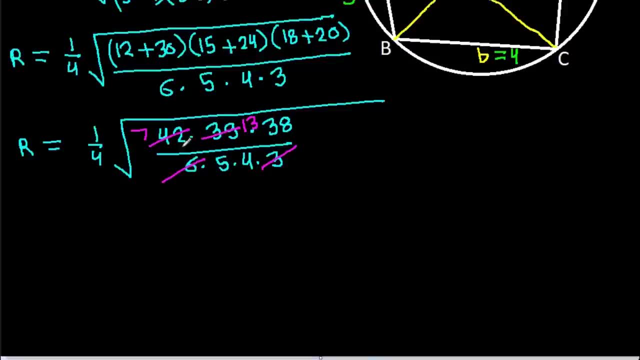 that is your 13 cd plus a. through the 15항 x 15 times 7 is 42 and 2 times 2 is 4, 2 times 19 is 38. So R it is 1 by 4 times a. 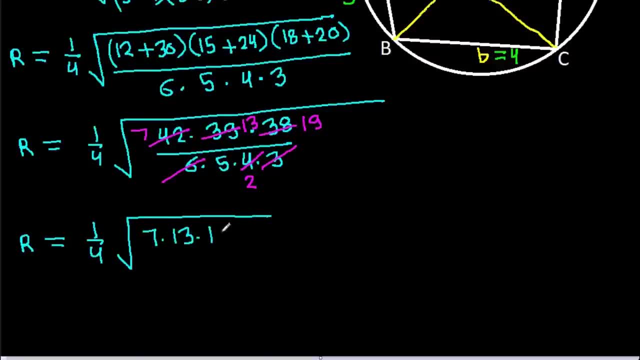 square root of 7 times 13 times 19. by 5 times 2 and 7 times 13 times 19, it is 91 times 19. that will be 91 times 20 minus 1 and it will be 1820 minus 91 that.